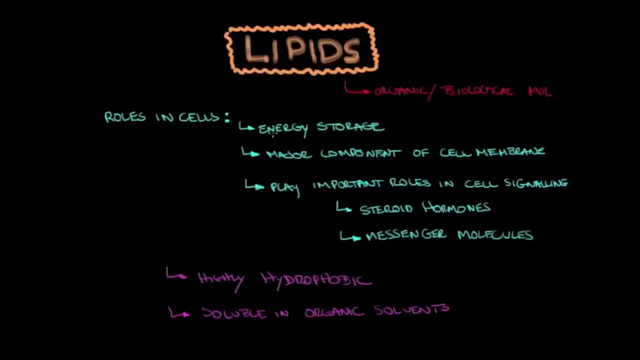 cells, And the first role is that they are energy storage molecules And if you look at lipids, they're able to form and break bonds, And when they do so, they're able to either release or store energy, And you're going to learn about that in more detail in. 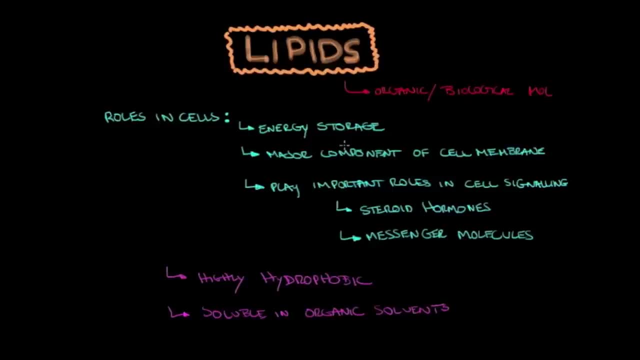 classes such as biochemistry, But for now have an idea. The second thing to know is that they're major components of cell membrane, And if I draw a cell here, I'm not a good artist. But anyway, what I want to have here is a simple drawing of. 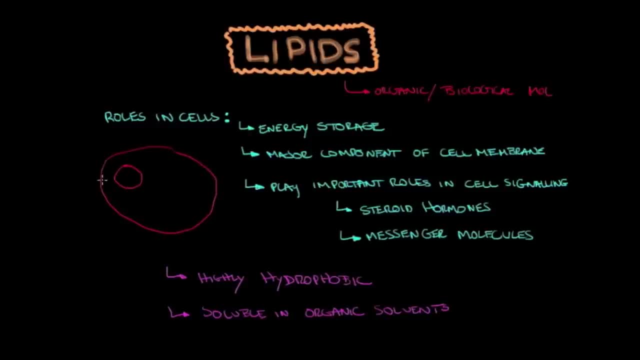 a cell with a nucleus, And this structure here surrounding my cytoplasm is called a cell membrane, And the cell membrane is comprised of a cell membrane. And the cell membrane is comprised of many things, including a phospholipid bilayer, And a phospholipid bilayer is: or a phospholipids. 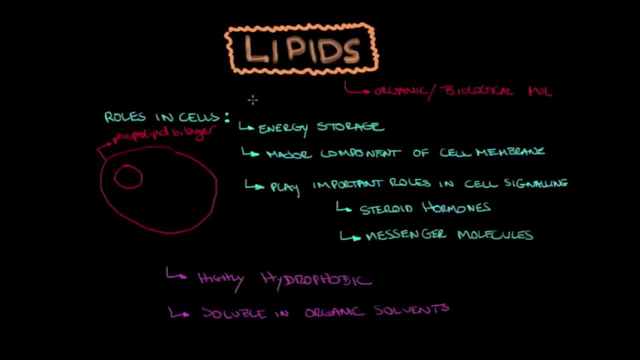 are clearly in this group, in this class of molecules, the lipids, And we're going to learn in a little bit more detail. We're going to talk about this structure, the cell membrane. You're going to see what I'm talking about, But for now, understand that this really, really important. 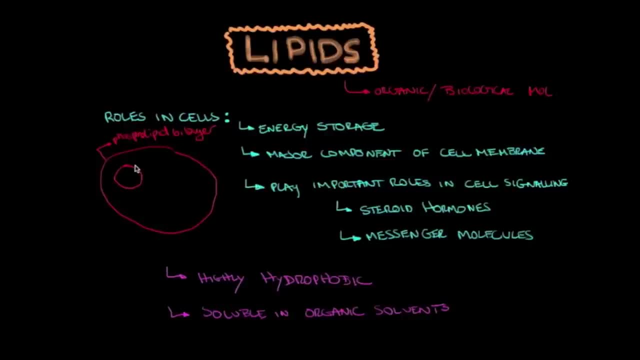 structure that surrounds the cytoplasm, that encloses the cytoplasm, is comprised of mainly lipids. Okay, The third thing that I want to talk about, the third role that lipids have, is in cell signaling. And what is cell signaling? Think about, cells need to communicate with one. 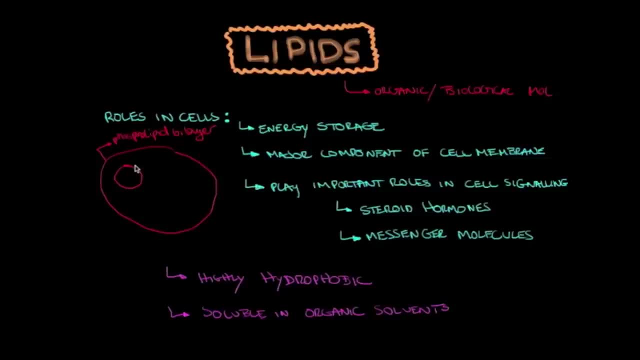 another. Because if there is a change in the outer environment, for example, cells need to adapt, let's say, in a way they need to cope with that change in the environment, And they do so by communicating with one another. They send these molecules that, let's say, warn them. 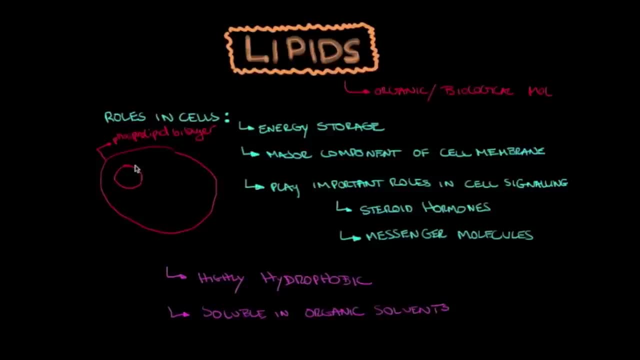 of the change of the environment And that way they're able to change their inner environment and, that way, cope with what has changed in the outer environment. Okay, This is a very simple way to think about cell signaling, And we're going to talk about it later in other tutorials. 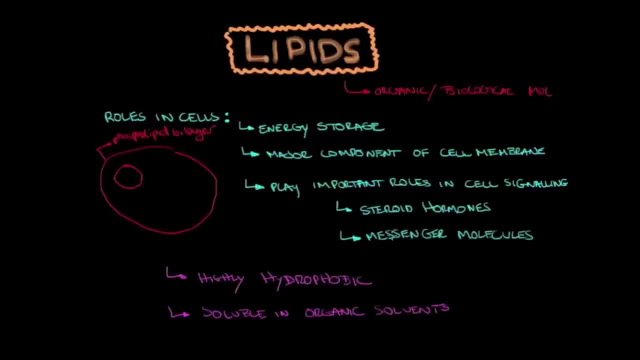 But for now know that Lipids are part of the structures of the molecules that are used as messenger molecules between these cells. They use these molecules to communicate with one another And there are some called steroid hormones, And steroids are definitely lipids And they have a very 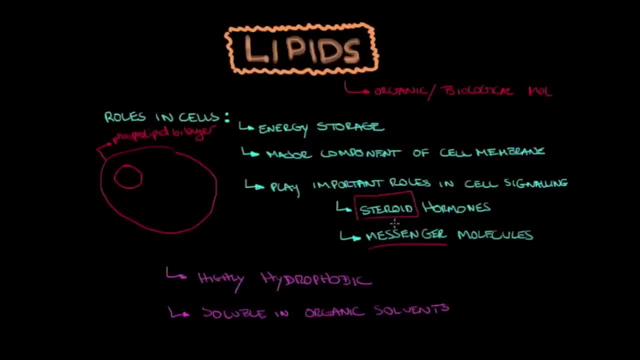 interesting structure that we are going to discuss also later on in this tutorial, called sterine. It's a very cool structure. You're going to learn a little bit about it. We're going to learn a little bit about it And we're going to talk about it later in this tutorial. 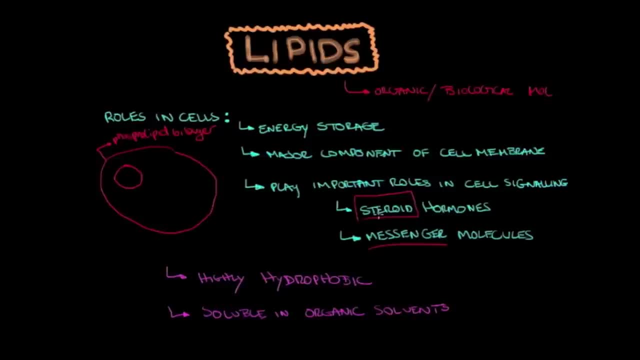 But for now, just keep in mind that there are steroid hormones which are used in cell signaling, And steroids are definitely lipids. Two last things I want to talk about lipids in this slide is that they're highly hydrophobic, And you probably know the definition of hydrophobic. 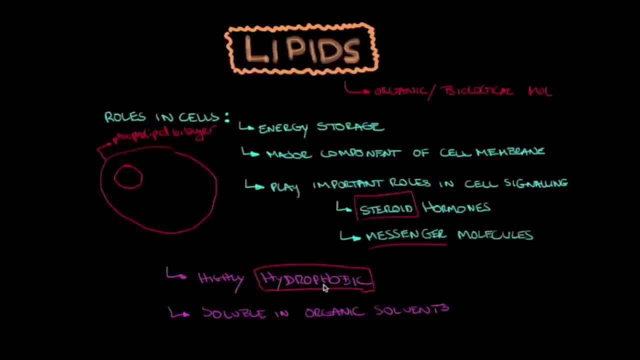 Hydrophobic means that doesn't like water, And to say that lipids do not interact with water molecules. well, And if you look, this is basic chemistry. But if you look, water is a great solvent. And why is it a great solvent? Because it has a positive side and a negative side. So 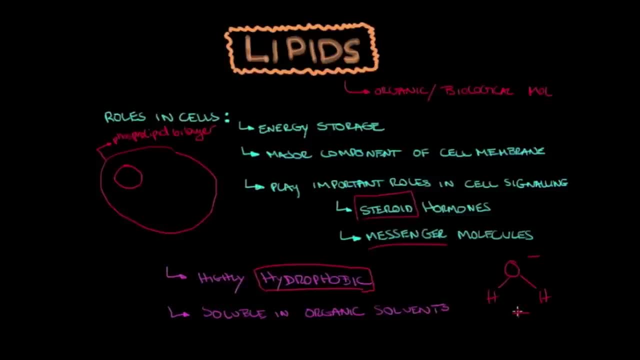 it's quite polar and it's able to interact with other polar molecules. But lipids have a very- not I was going to say weird, but not weird- structure. They're comprised of long chains of carbons which make them kind of non-polar. 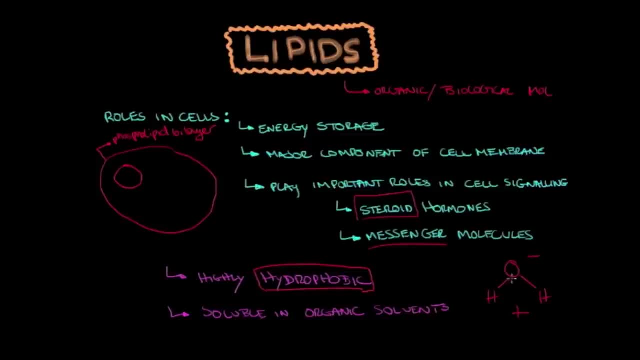 And because they're non-polar, they can't interact. They don't have the negative or the positive side where water molecule- or, yeah, water molecules- can go in and interact and be, you know, the solvent for this type of molecules. That's why they're only soluble. 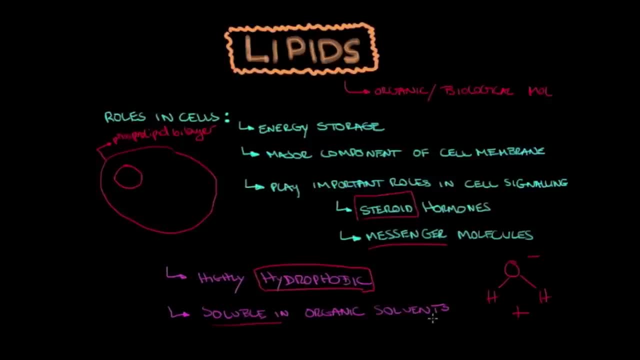 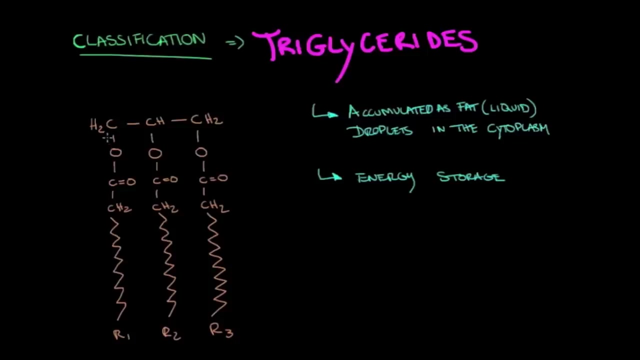 soluble in organic solvents, And organic solvents are definitely non-polar, So, and that's why they interact well with lipids, because lipids are also non-polar due to the long chains of carbons. So I talked about lipids and I gave you a basic description of what these 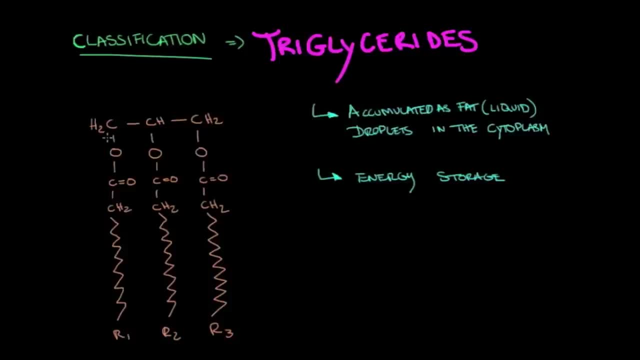 molecules are But for biology or molecular and cellular biology. I want to give you just the basic description or classification of these molecules, And you can find different ones out there for lipids, And the first one I want to talk about is triglycerides. 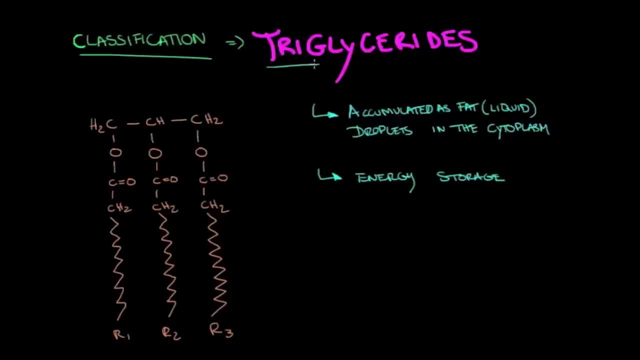 And, as the name indicates, Triglycerides, meaning we're going to see three things, and the three things we're going to see are these three fatty acids that you find here. So these are three fatty acids and they're going to be bound to this structure here, which is called 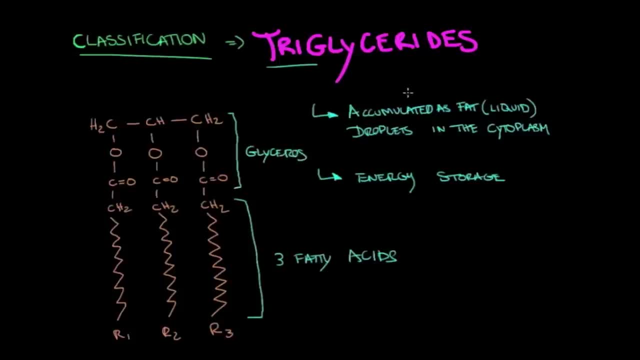 a glycerol molecule. So what triglyceride is – sorry, let me – its glycerol? So a triglycerides? Triglyceride is three fatty acids bound to a glycerol molecule, as you can see here. 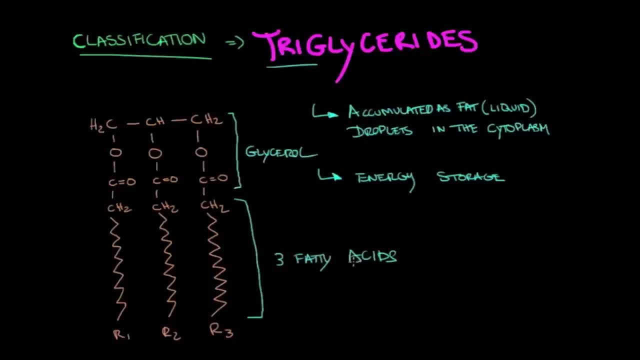 And these three fatty acids and look at your organic chemistry notes, because you're going to see some more detail there. but for biology purposes, all I want to say about these fatty acids is that they can vary. That's why I put different names here, different letters and numbers- R1,, R2, and R3, because 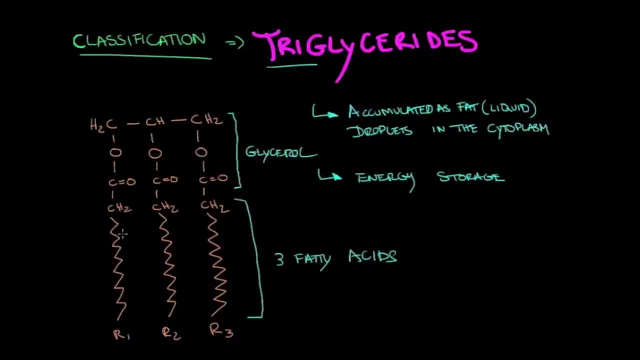 they can definitely vary according to the oil, according to the bonds between these long carbon chains. here They can have saturated or unsaturated molecules, and you can see that in more detail in your organic chemistry notes. But for now just keep in mind that triglycerides are these glycerol molecules that bound to 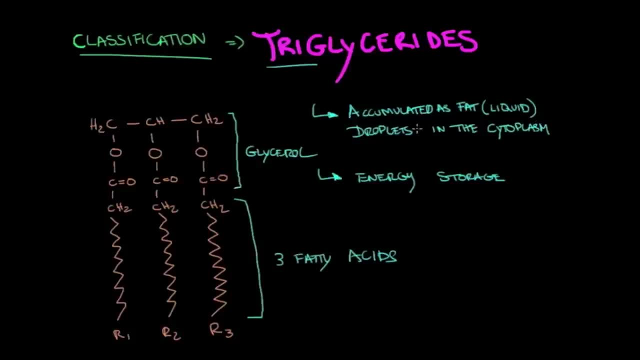 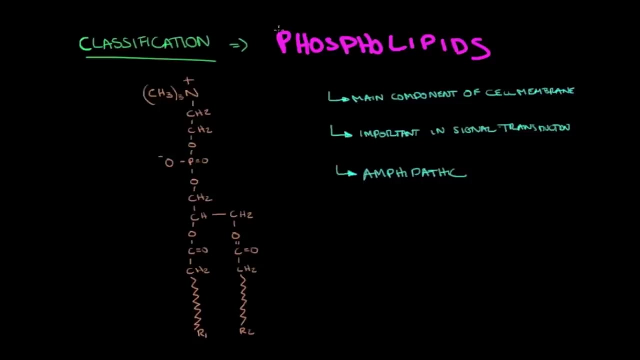 three fatty acids, And these are seen in your cells. accumulated acids, That's fat liquid droplets in the cytoplasm of your cells, and this is how energy is actually stored. It's time to talk about phospholipids, and I have a representation of these molecules. 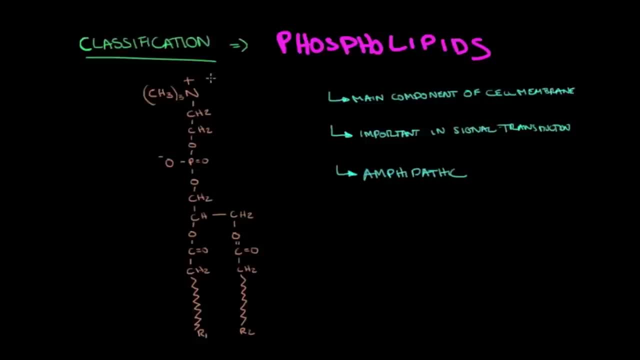 right here on the left and it looks complicated, but it's not. What you are seeing here is a choline. so this is a choline, and then you find a phosphate group. It's right here, and the phosphate group is attached to the third carbon. on the glycerol. 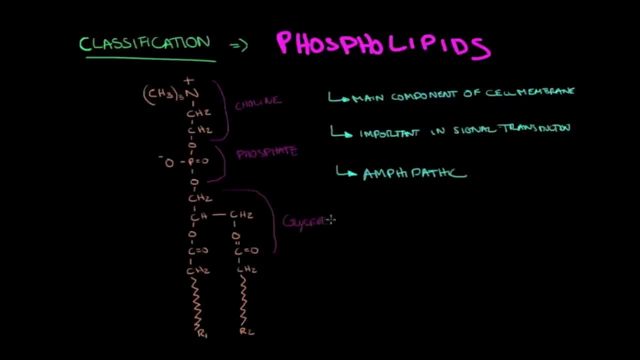 molecule. so this is a glycerol molecule and you saw a glycerol molecule attached to three fatty acids in triglycerides. but on phospholipids you're going to find only two fatty acids and the third carbon of the glycerol is here. 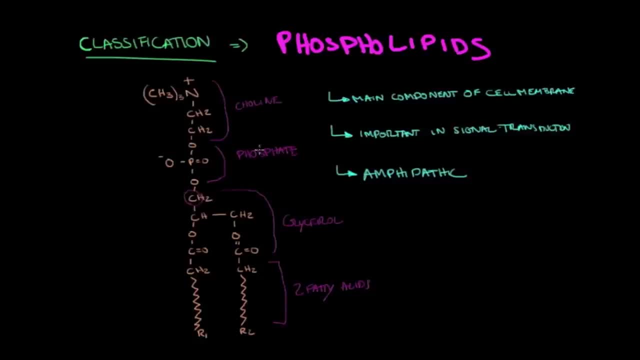 This is the carbon that is bound. The third carbon is bound to the phosphate group and because this happens, you see a phosphate group attached or bound to a glycerol molecule. These can also be called glycerophospholipids. 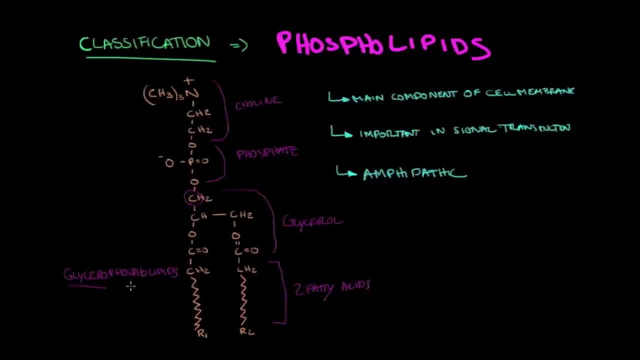 Makes sense, right? You see a glycerol molecule bound to a phosphate group, and what I want to also explain here in the phospholipids Is that from basic biology, where you learn that the basic structure or the simple way, 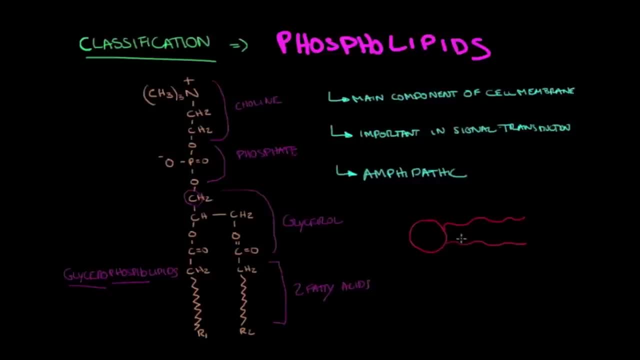 to represent a phospholipid is a one head attached or bound to two tails, which is what we see here. Say, this is the head right here, okay, it would probably include the glycerol, but anyway. and then you have the two tails and what I can show you on this head and two tails. 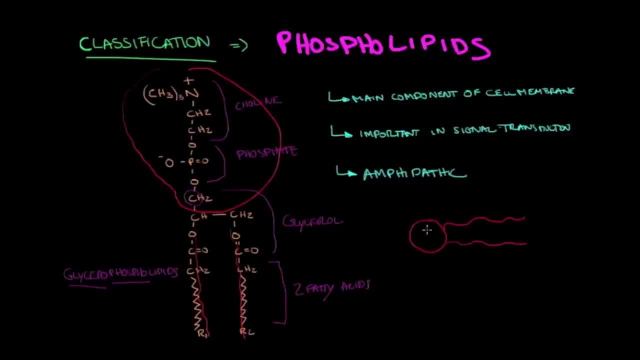 is that You find in or on the head. you find a positive charge right here and a negative charge, So one positive and one negative side of the head of my phospholipid and that means that this side is hydrophilic, meaning that because you find two charges here, it's going to interact. 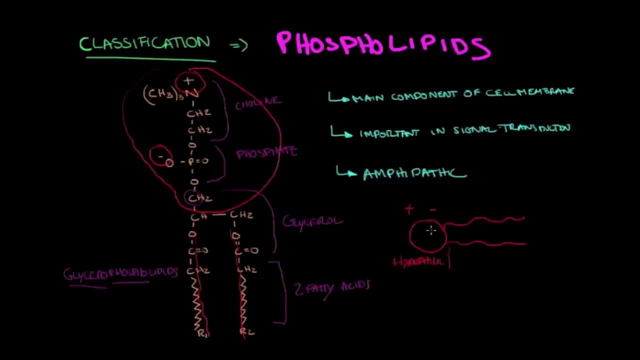 very well with water, because water also has two charges, one positive and one negative on the oxygen. This is basic chemistry, Again with basic organic chemistry. you know that because of the fatty acids- and the fatty acids are comprised of long chains of carbon atoms- you know that this part of the molecule 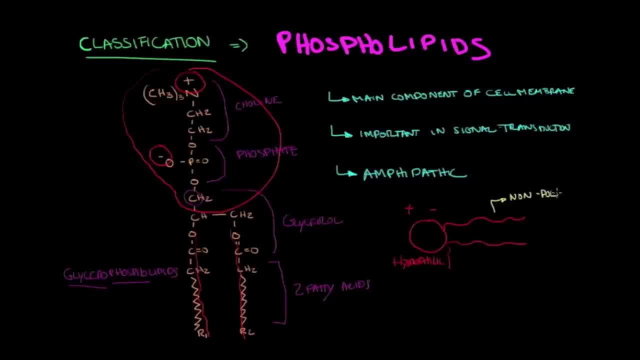 here is non-polar And because it is non-polar This is hydrophobic, meaning that it does not interact well with water. Say, a water molecule comes in with two charges. let's say I'm going to draw my water molecule. 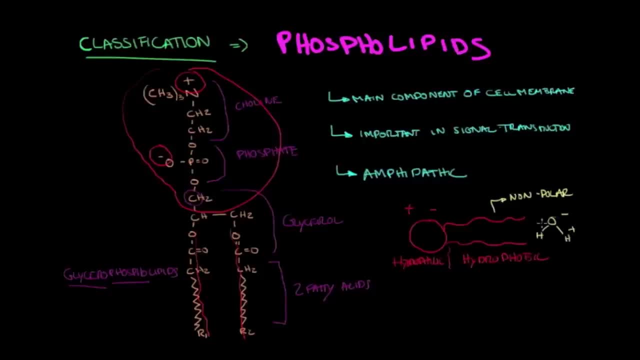 here with a negative charge and a positive charge comes here, does not see any any charge to interact with, only in this side in the head where you find a positive and negative charge. Therefore, it will not be able to interact at all. 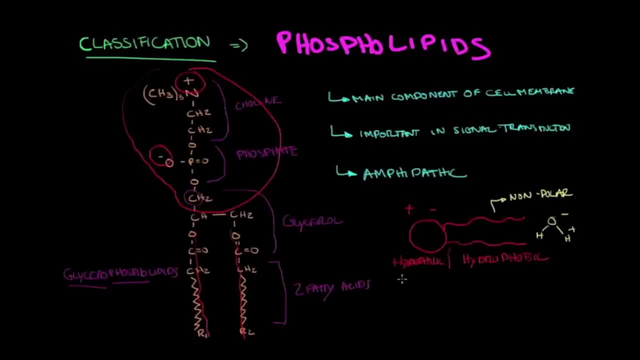 That's why- because you find a hydrophilic and hydrophobic side on this, on only one phospholipid- you call these molecules amphipatic. They're able to do both things. They're able to be hydrophilic and hydrophobic, like amphibious or amphibians who are able. 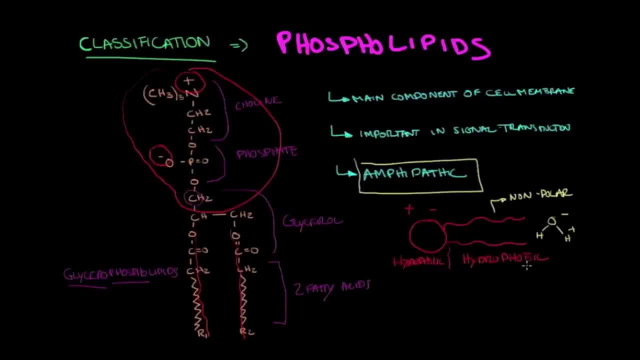 to walk on land and live in water. They're able to do both things. They're able to be hydrophilic and hydrophilic like amphibious or amphibians who are able to walk on land and live in water. So these molecules are able to do two things, two opposite characteristics- okay. 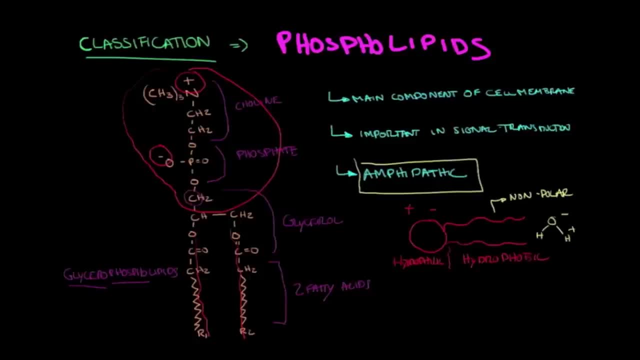 Another thing I want to mention is that the main component of the cell membrane is phospholipids. So if you look at a cell- again, my beautiful cell here with a nucleus, this area here enclosing the cytoplasm, which is the cell membrane, is comprised of a phospholipid bilayer and 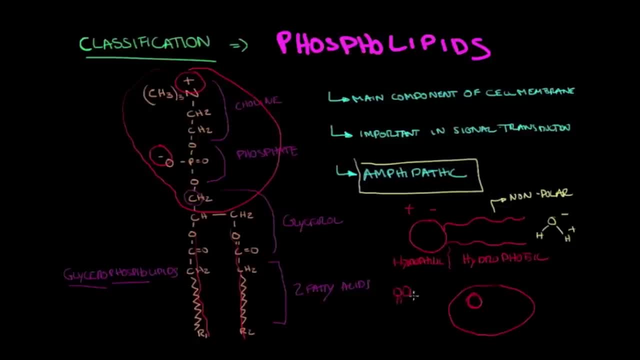 by phospholipid bilayer. you're going to learn that in more detail. I'm going to show you in a different tutorial. but a phospholipid bilayer, you see all of these structures, but in two layers. So this is why bilayer- again word origin- and this is what you find in this area here. 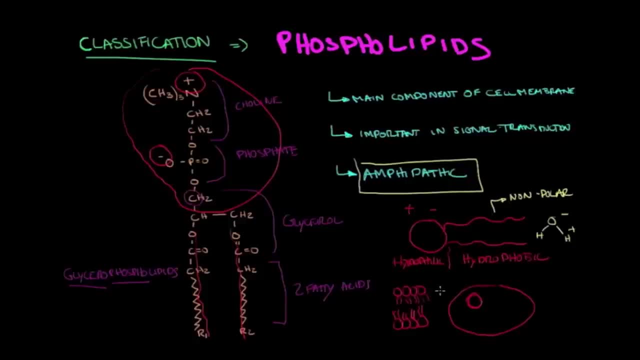 in the cell's membrane And you will also see other structures like proteins and carbohydrates, but the main component is definitely phospholipids. Second thing to mention to talk about phospholipids is that they're important in signal transduction. 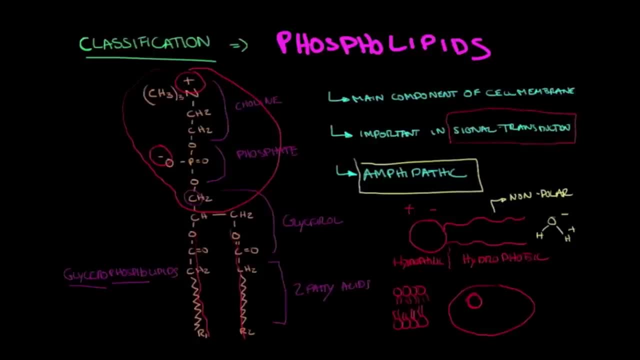 Signal transduction is when something happens in the environment and say there is stress caused or something is happening and there are signaling molecules in the environment which will interact with the cell's membrane and then it will produce some sort of signal And therefore a pathway is going to be ignited, let's say, or stimulated, let's say, inside. 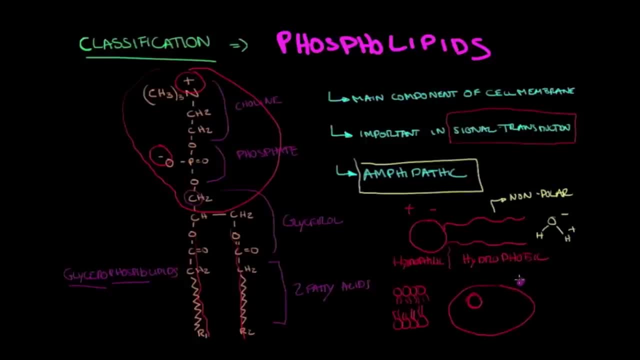 of the cell. So if you imagine a molecule interacting with the cell, the first layer that it's going to find, the first thing that it's going to have contact with, is definitely the phospholipid bilayer And therefore there is some importance involved in the signal transduction and we are going 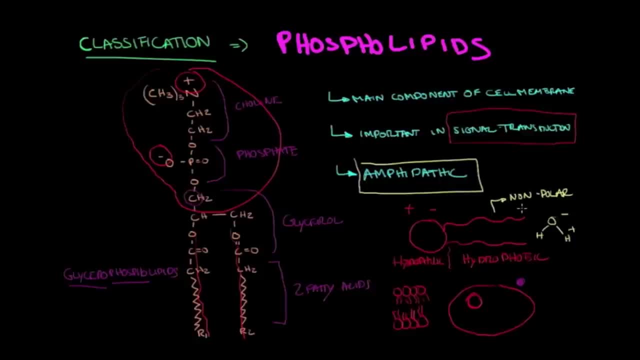 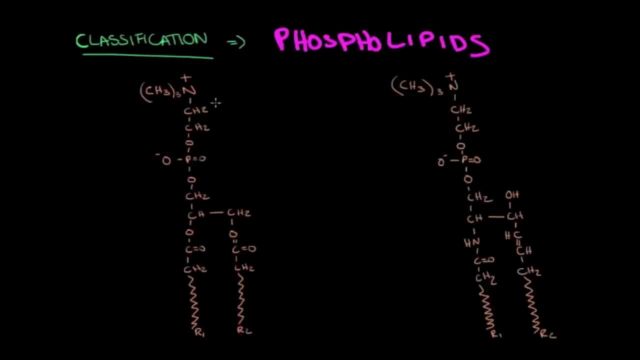 to see that later, But for now, keep in mind that phospholipids have, or play, an important role in signal transduction. I want to give a quick note on this one. We're still talking about phospholipids and the molecule. we have two molecules here. 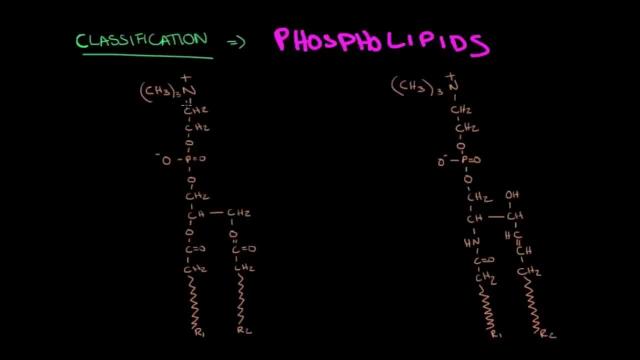 that need to be compared. very briefly, And the molecule you have on the left is a glycerophospholipid, like the one I talked about previously. So glycerophospholipid, So this is a no need for an S. so this is a glycerophospholipid, meaning that I have. 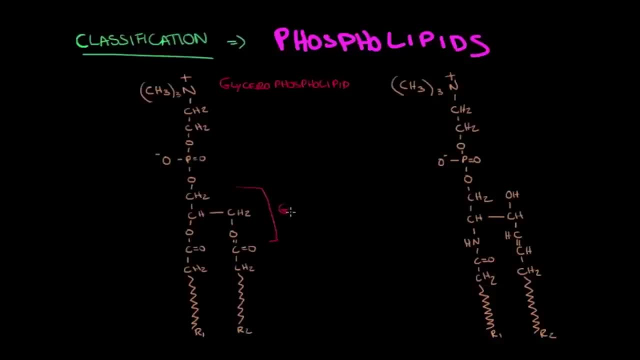 a glycerol molecule here bound to a phosphate group that you find here. So this is my phosphate. But there is another type of molecules that you can find in your cell's membranes, and these are called. they have an interesting name. 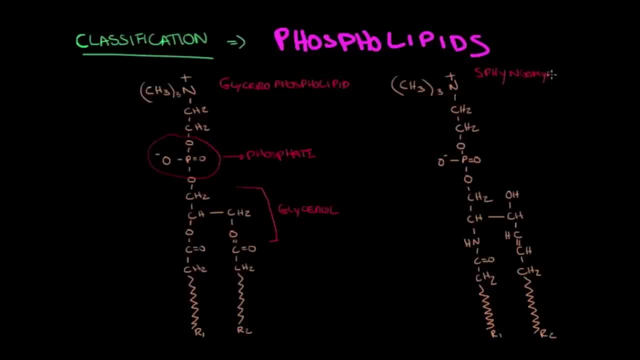 Vengomyelin. These are found in your cell's membranes, So other types of phospholipids found in your cell's membranes. And what happens here? the difference, the major difference between these two- you can still find a polar head here, because you have a positive side here and a negative. 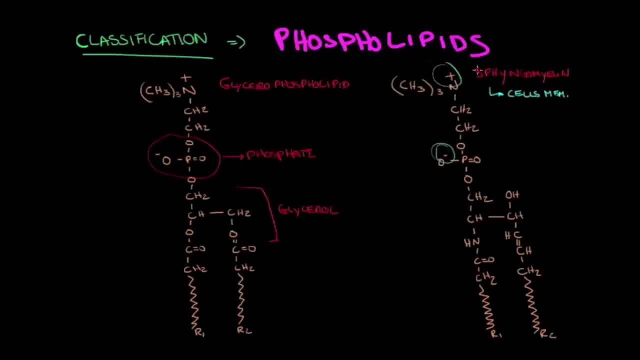 charge here. So So a positive charge and a negative charge makes that polar head. but instead of glycerol- you do not find a glycerol here. instead you find a. let me change to red. instead you find a serine molecule. 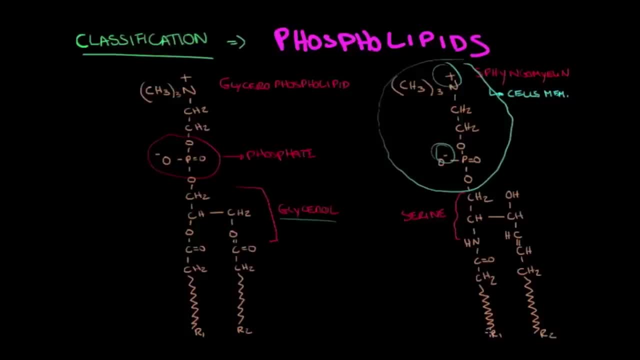 And this is where your fatty acids are attached to or bound to. and what happens here is that if you look at this structure here- Okay, So this structure here is called trying to draw here. this structure here is called a sphingosine. 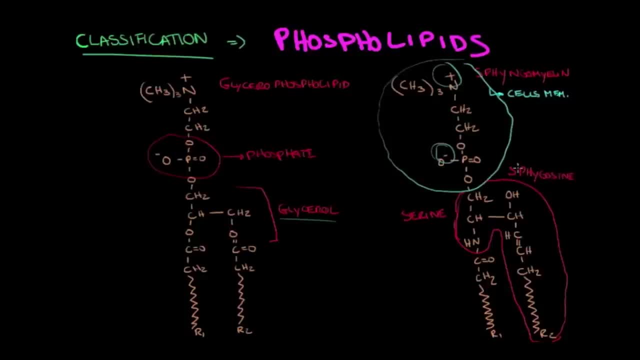 I'm just giving you nomenclature and explaining a little bit why you find why, or the importance of sphingomyelin in your cells quickly, Do you find them? It's a phospholipid And the major difference here is that. 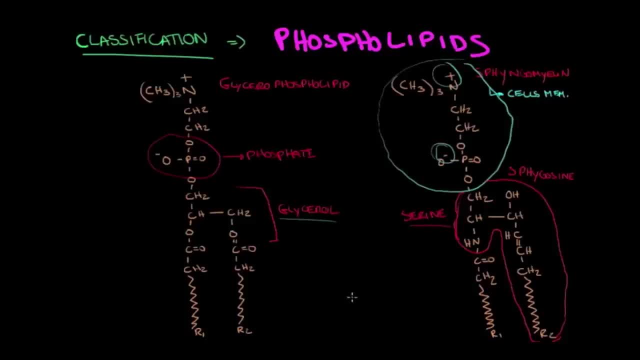 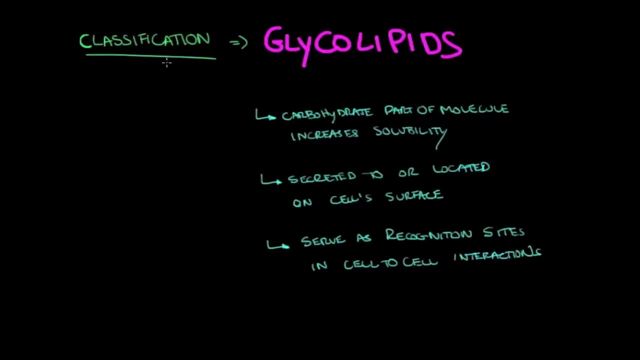 Okay, You do not see a glycerol molecule. instead, you find a serine molecule and these- this is where your fatty acids will bind to. Another class of lipids that we see out there on in your cells. are these called glycolipids? 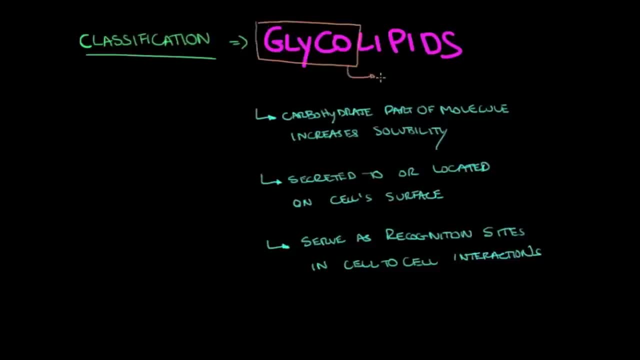 And glyco means carbohydrates or sugars. so you're going to find a carbohydrate or a sugar associated to a lipid And, as you know, sugars are good solutes. they dissolve very well in water and therefore, if you associate a carbohydrate to a lipid molecule, what you're going to do, you're. 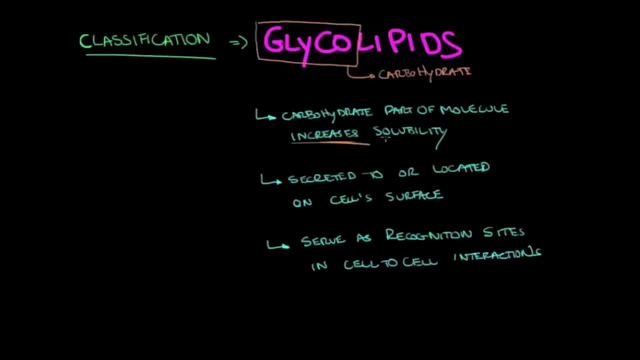 actually going to be able to increase the solubility of the molecule Because, as you know, lipids are not do not dissolve well in water, They're not good solutes in water. But if you associate a carbohydrate you can definitely increase that solubility. 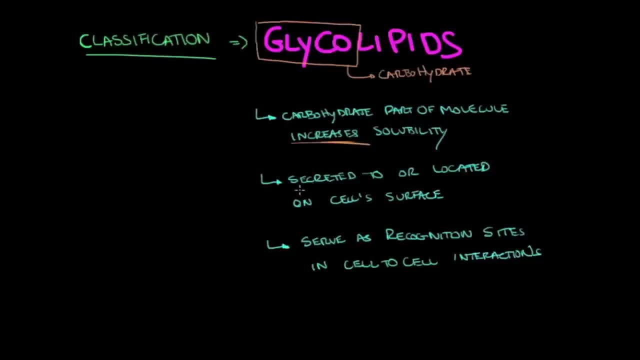 The second point I want to make on glycol lipids is that they are secreted to or located in the cell surface, And what I mean by this. if I have my cell here again, you can find these molecules somewhere on this area here. 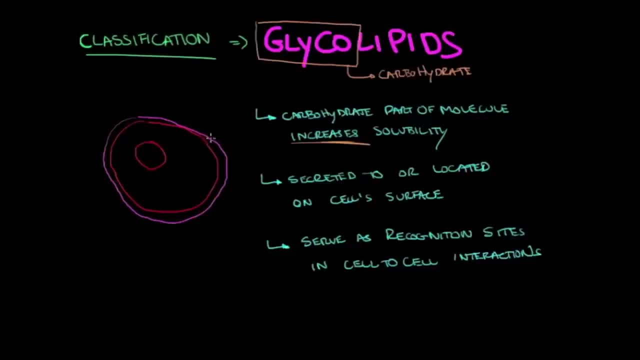 So the outside of the membrane, okay, located on the outside, not the inner part that is in contact with a cytoplasm, but the outside of the membrane, The membrane that is in contact with the outer environment. okay, This is where you find glycol lipids. 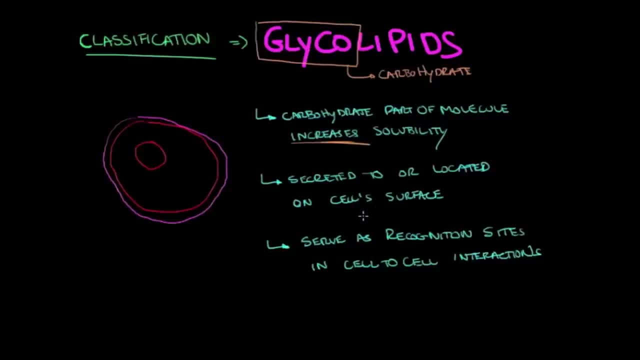 And it actually is associated to the function of these molecules because they work as markers or they serve as recognition sites in cell-to-cell interaction. So they work as markers, And what this is is that these molecules are able to work or to be um, so they can. 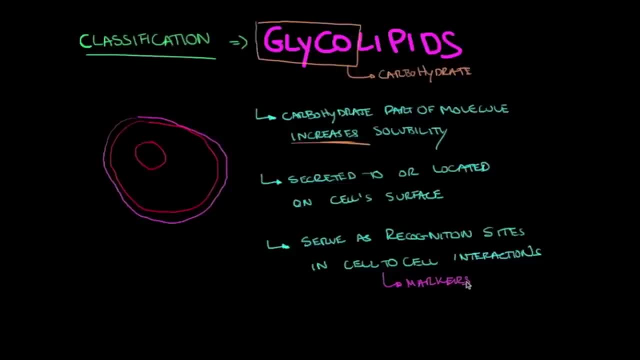 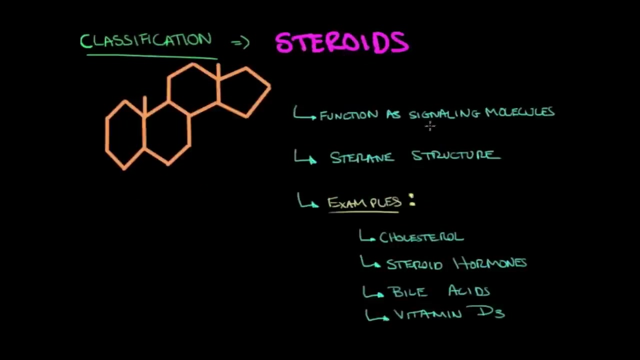 use some sort of code, I would risk to say that is used in this type of interaction And that's why we call it markers. Now let's talk about steroids. Steroids are definitely lipids, okay, And they function as signaling molecules in your cells. 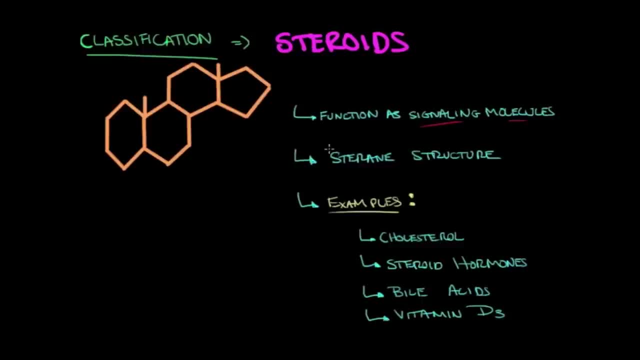 And I have a basic structure of a steroid, which is the sterine structure. They have this common structure And what happens is that A sterine, sorry structure is comprised of three cyclohexanes, meaning three six-carbon rings. 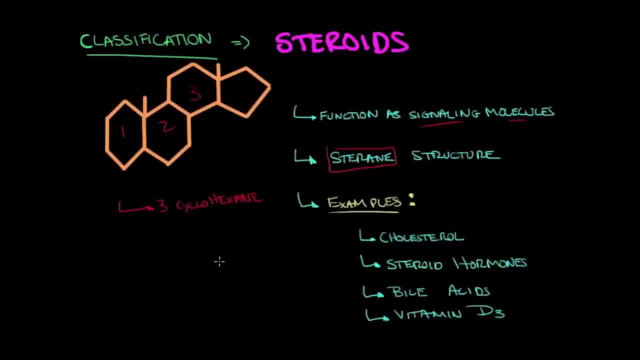 So one, two and three, Six carbon rings And one cyclopentane, meaning one five-carbon ring, And this is my one, So I'm going to put one Cyclopentane with five carbons, so a five-carbon ring. 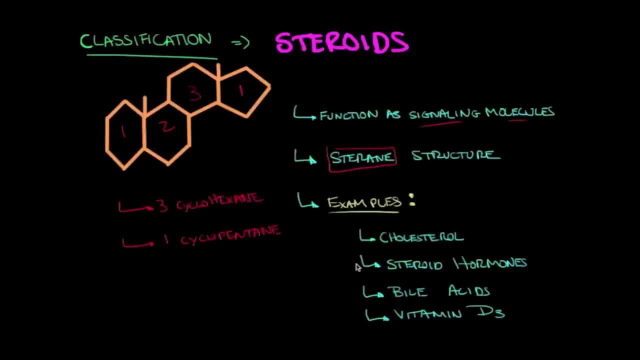 And examples of steroids. you can find them in many forms, but they all have this sterine structure. keep that in mind. But the forms or the examples you can find steroids are cholesterol, steroid hormones, for example, testosterone is a steroid hormone. you have testosterone, sorry, is a steroid.